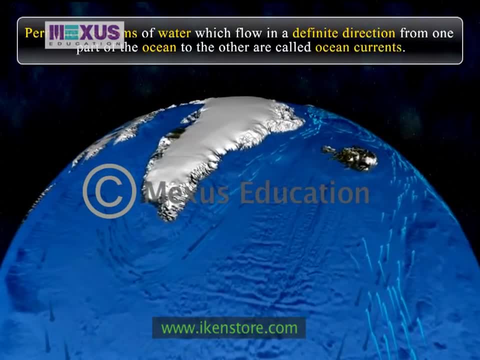 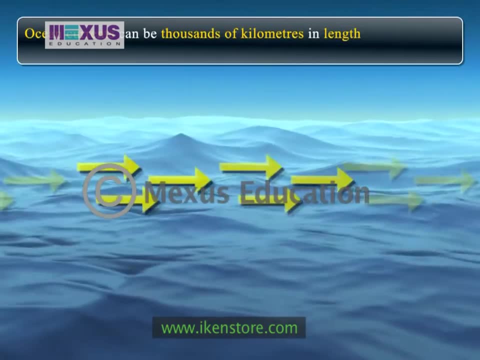 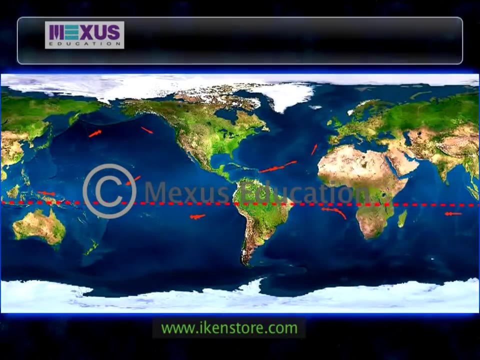 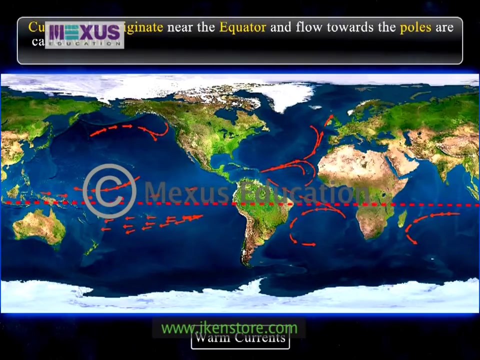 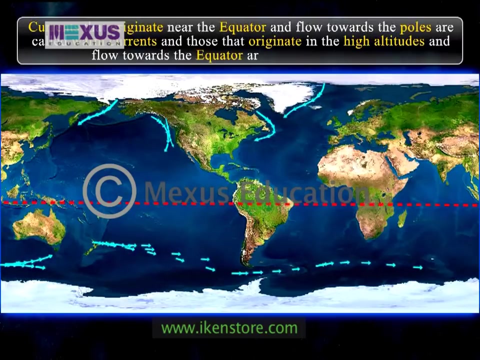 to the other are called ocean currents. Ocean currents can be thousands of kilometers in length and sometimes about 200 kilometers wide. Currents that originate near the equator and flow towards the poles are called currents, Warm currents, and those which originate in the high altitudes and flow towards the equator are 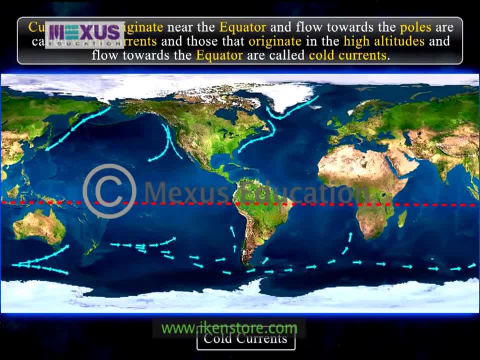 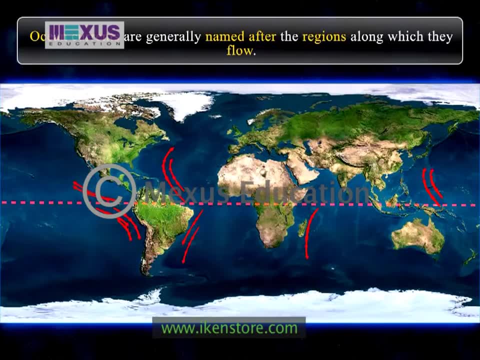 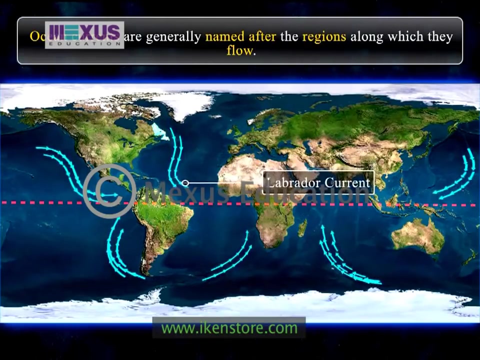 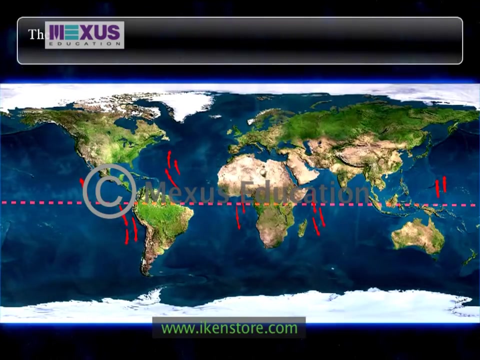 called cold currents. Ocean currents are generally named after the regions along which they flow. The warm ocean current flowing along the Brazilian coast is called the Brazilian current and the cold current flowing along the Labrador coast is known as the Brazilian current, Also known as the Labrador current, the Safora and the Balan. 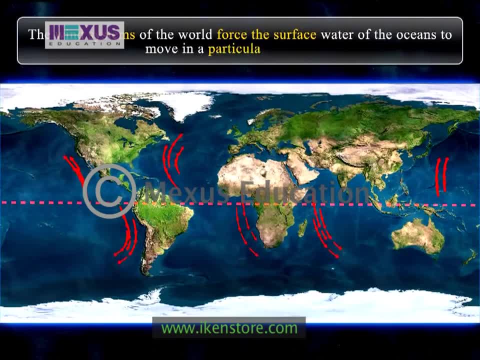 currents move on the coast, smoothen the waters and predict the future of the experiment. Ocean currents are powered by the wind system of the world. The wind systems of the world force the surface water of the ocean to move in a particular direction: a surface current of warm and light. 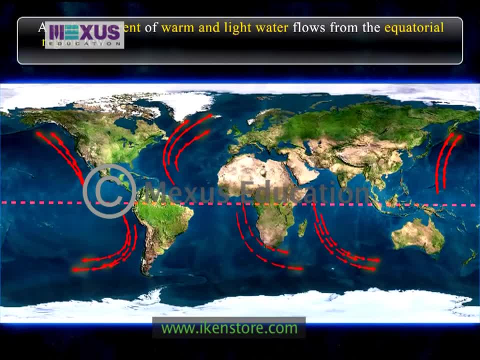 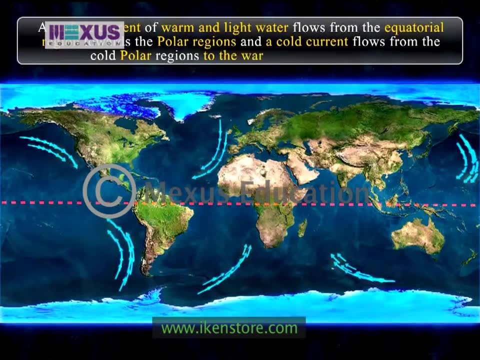 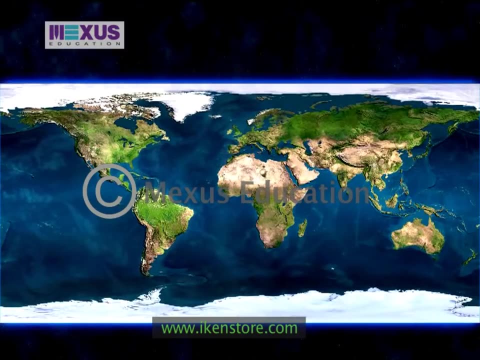 water flows from the equatorial region towards the polar region and a cold current flows from the cold polar regions to the west, And these currents provide cool water. and that's what we are talking about. as you know, the warm equatorial region. The prevailing winds lend speed and direction to a mass of water. 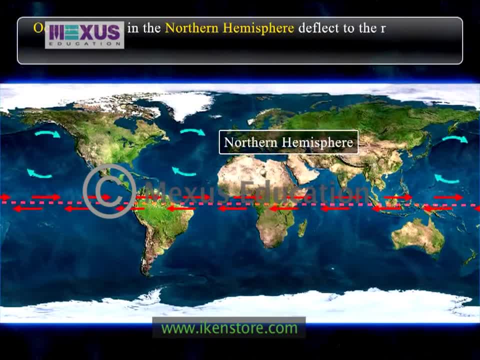 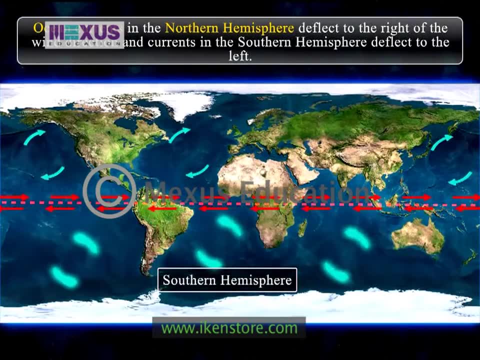 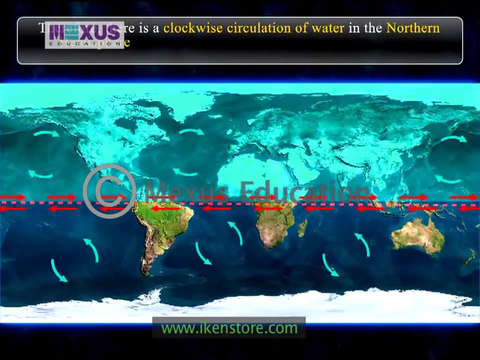 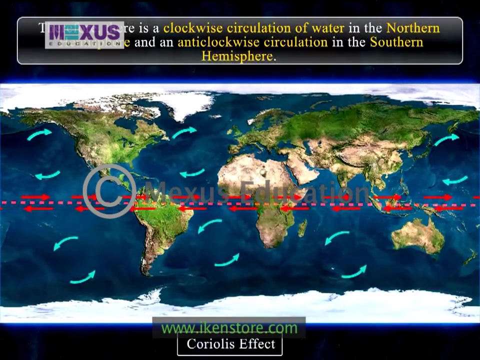 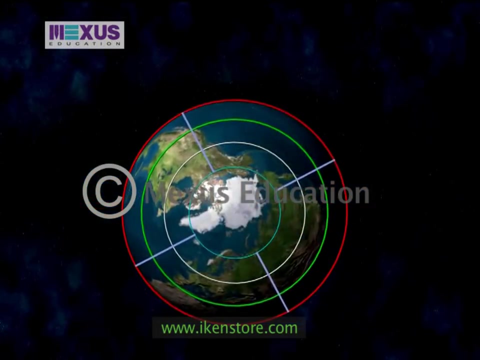 Ocean currents in the northern hemisphere deflect to the right of the wind direction and currents in the southern hemisphere deflect to the left. Therefore, there is a clockwise circulation of water in the northern hemisphere and an anti-clockwise circulation in the southern hemisphere. This is a Coriolis effect caused due to the rotation of the Earth. 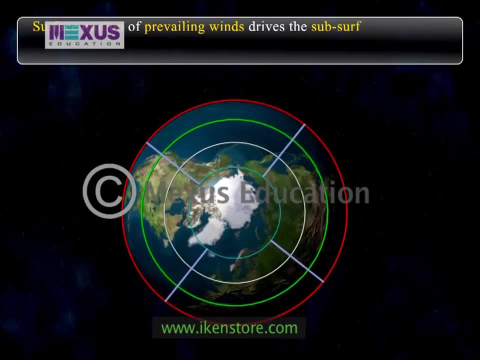 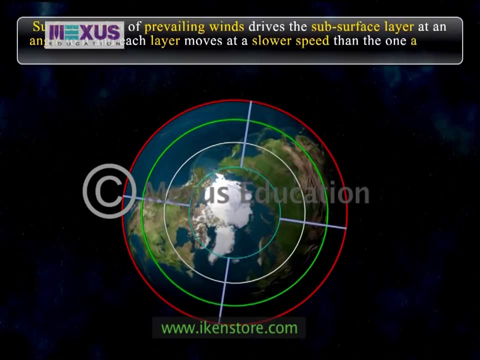 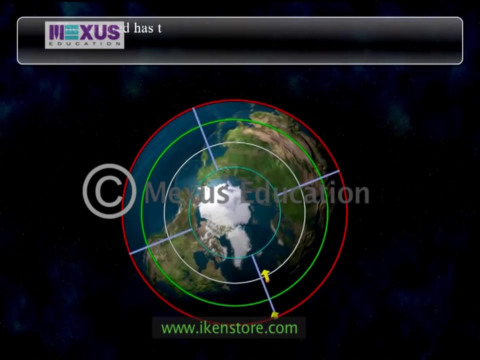 Surface motion of prevailing winds drives the subsurface layer at an angle to it. Each layer moves at a slower speed. Each layer moves at a slower speed than the one above it and at a greater angle from the wind. The spiral thus created has the overall effect of moving the water mass above the depth of. 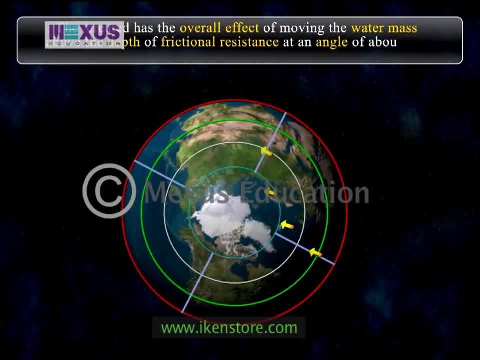 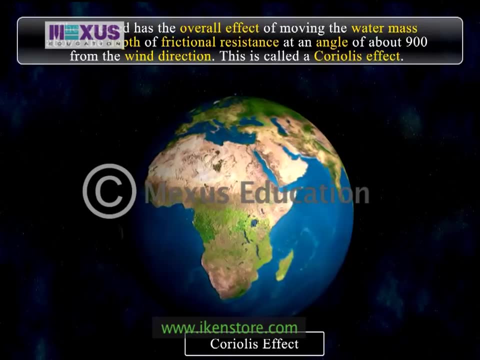 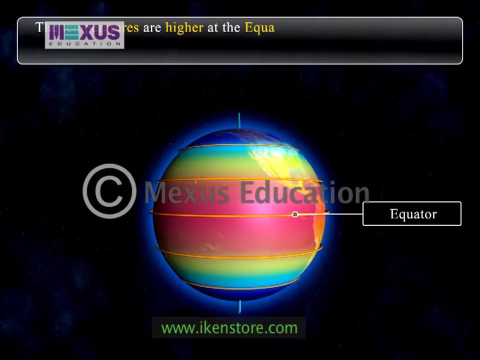 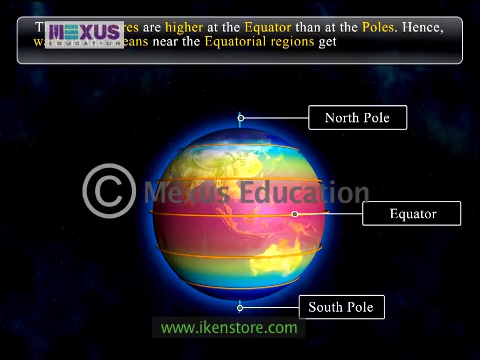 frictional resistance at an angle of about 900 from the wind direction. This is called a Coriolis effect. The temperatures are higher at the equator than at the poles, Hence water in the oceans near the equatorial regions gets heated more than the one in the 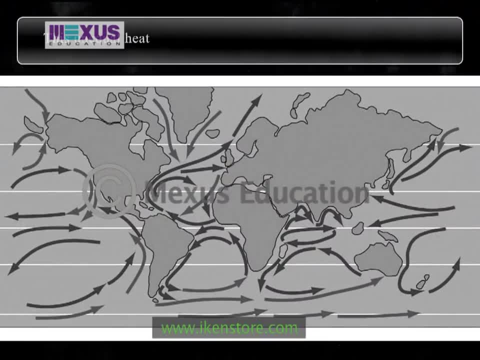 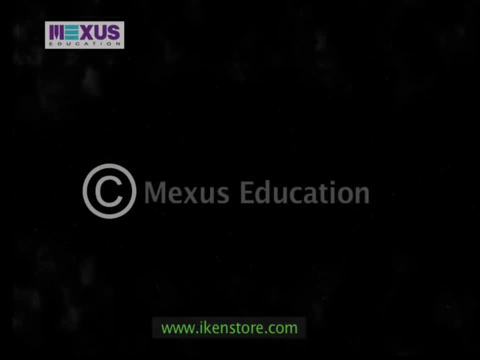 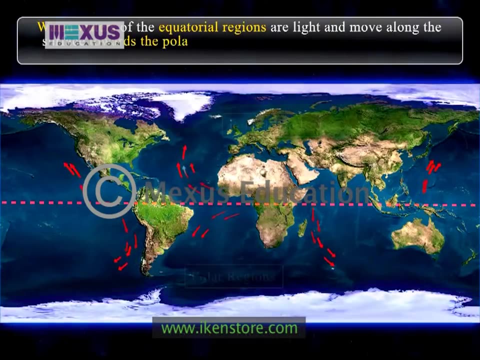 oceans near the poles. This unequal heating sets up convectional currents in the ocean. Warm waters of the equatorial regions are light and move along the surface towards the equator. They move towards the polar regions where they are cooled, while the cold water is dense. 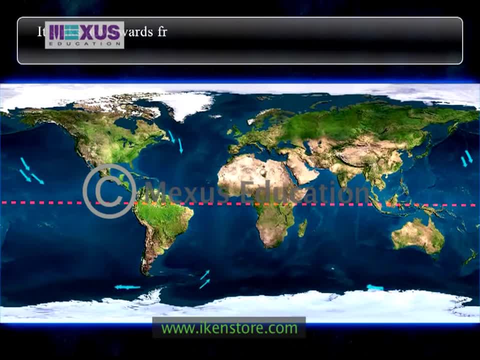 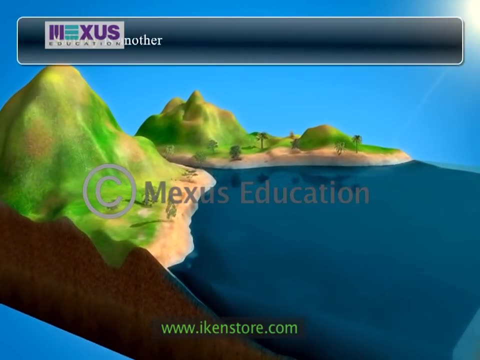 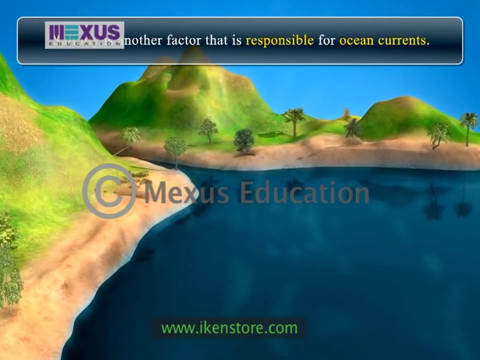 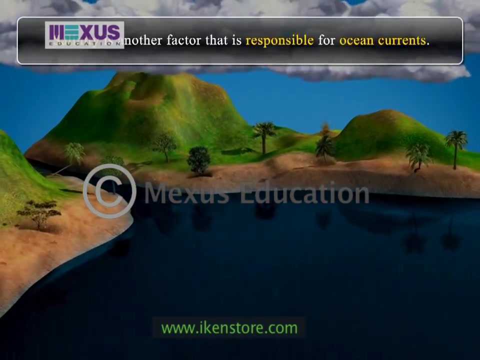 and heavy. It sinks downwards from the surface and moves slowly towards the equator, where, on warming up, it may rise to the surface again. The temperature of the polar regions is determined by the inflow of fresh water from rivers, melting ice and rainfall, as well as evaporation. 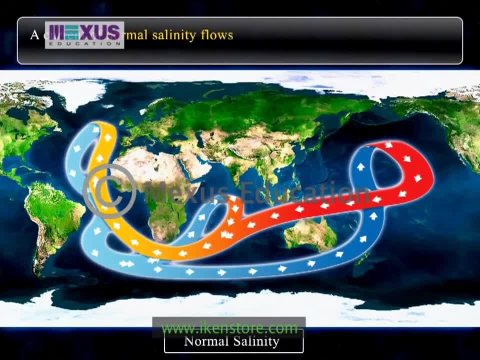 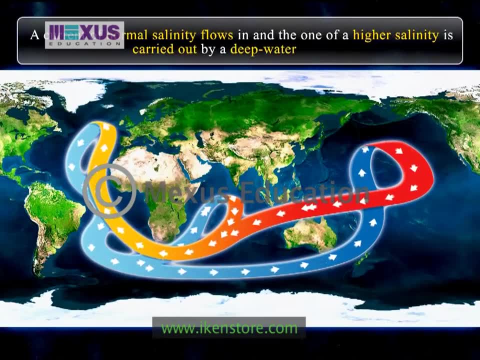 A current of normal salinity flows in and the one of a higher salinity is carried out by a deeper water current. For example, a high rate of evaporation in the Mediterranean Sea is determined by the current of the sea increases the salinity and therefore the density of the water. 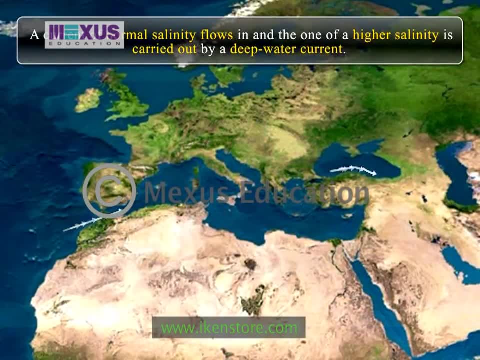 As a result, a current of less dense- that is, less salt- water flows into the Mediterranean from the Atlantic and the Black Sea, while smaller currents of higher salinity flow outwards beneath these currents, so that the salt content of the basin remains constant. 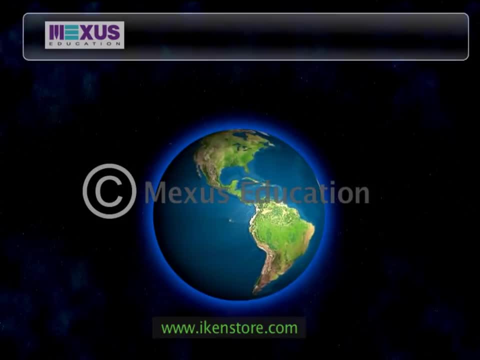 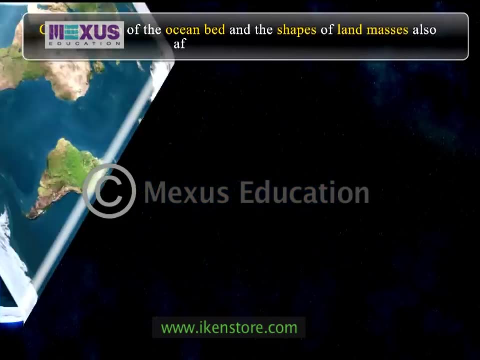 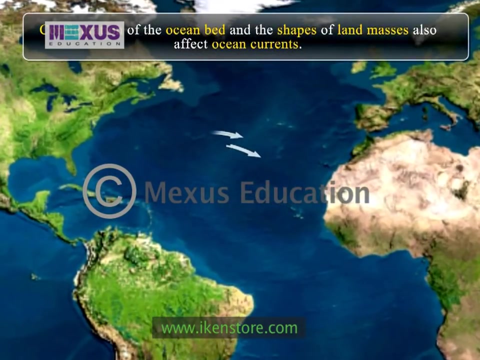 Other factors affecting currents are the configuration of the ocean bed and the shapes of land masses. For example, in the Atlantic Ocean, the North Equatorial Current flows towards the West Indies. Most of the current is channeled into the Gulf of Mexico. 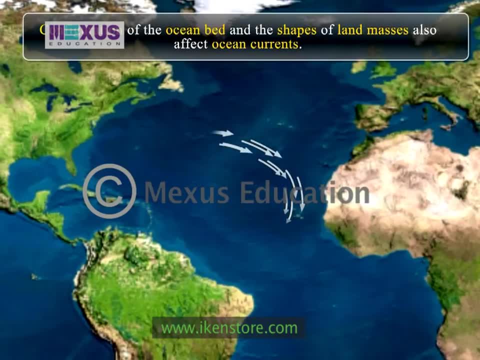 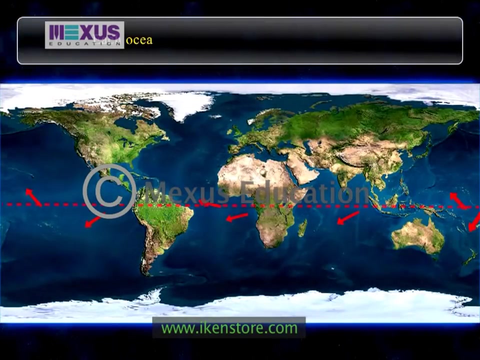 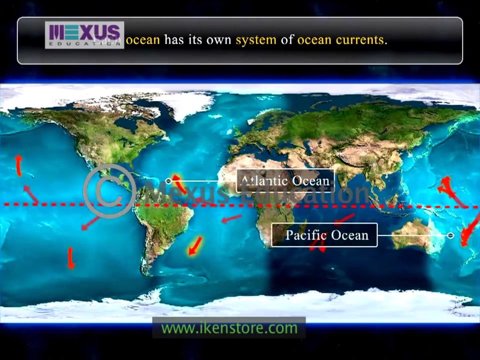 where it veers northeastward, bursting into the Atlantic Ocean between Florida and Cuba. Each ocean has its own system of ocean currents. The ocean currents of the Atlantic Ocean and Pacific Ocean show a common pattern. Ocean currents originate in the equatorial ocean. 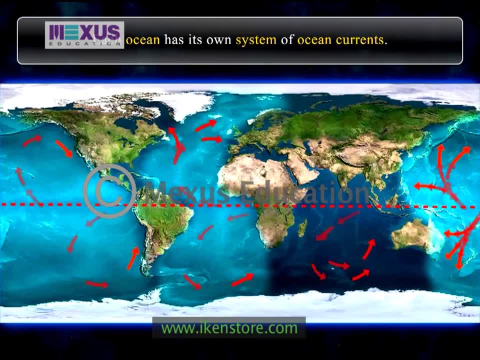 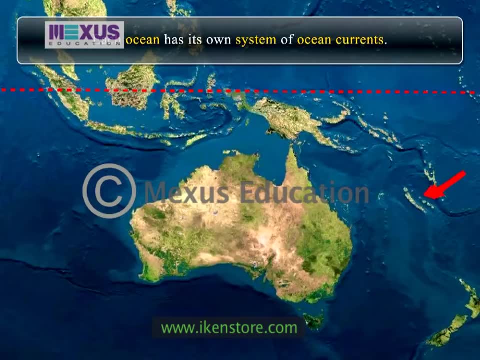 as the warm equatorial currents and flow westward. When they encounter continents, they divide into two branches. One is deflected northwards and the other southwards. These warm currents move along the east coast in the low and middle latitudes. 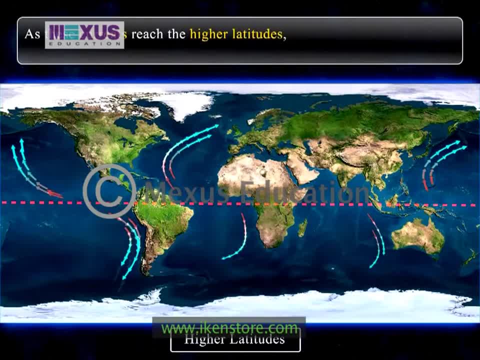 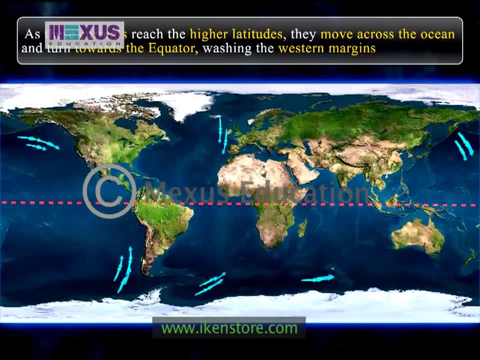 As these currents reach the higher latitudes, they move across the ocean and turn towards the equator, washing the western margins of continents. But this time the warm current loses much of its warmth and flows along the west coast as a cool current. 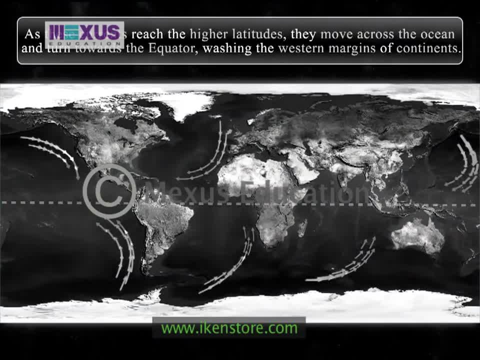 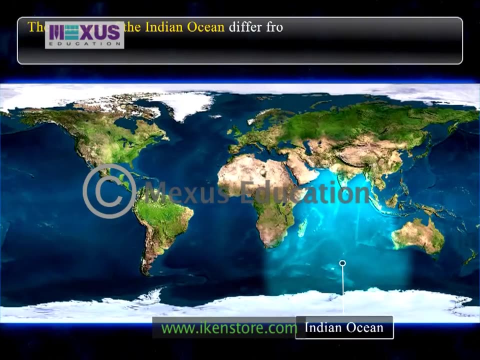 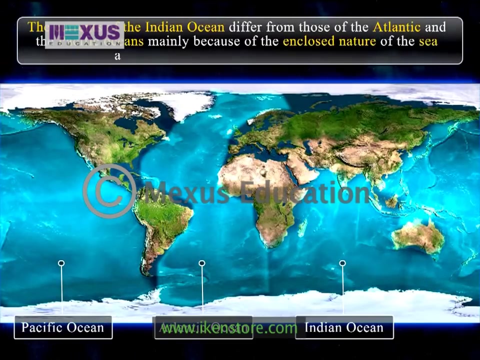 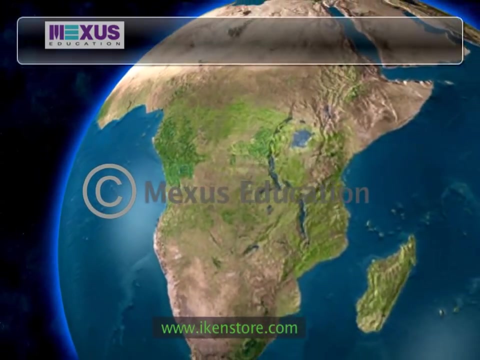 Finally, the current warms up as it reaches the equator and becomes a part of the equatorial current. The currents of the Indian Ocean differ from those of the Atlantic and the Pacific Oceans mainly because of the enclosed nature of the sea and the influence of the monsoon winds. 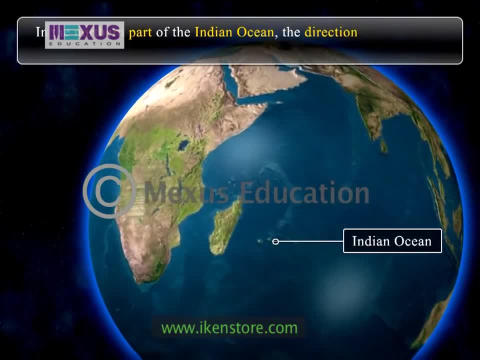 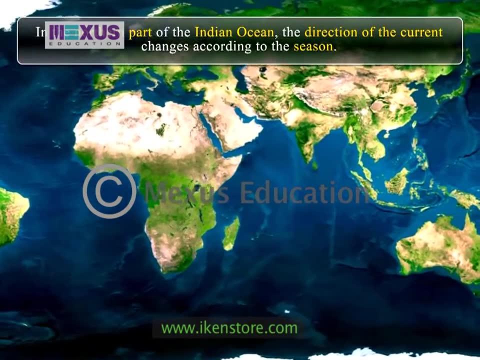 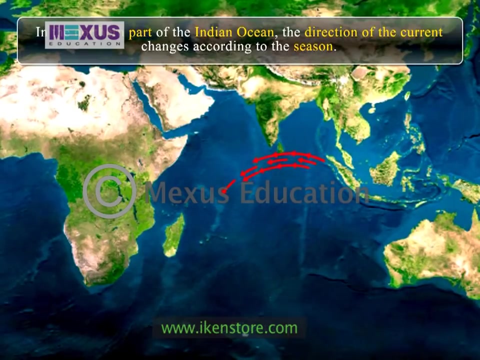 In the northern part of the Indian Ocean. the direction of the current changes according to the season: In summer, when southwest monsoons blow, the current flows in the western direction, And in winter, when the northeast monsoon winds blow, the current flows in the eastern direction. 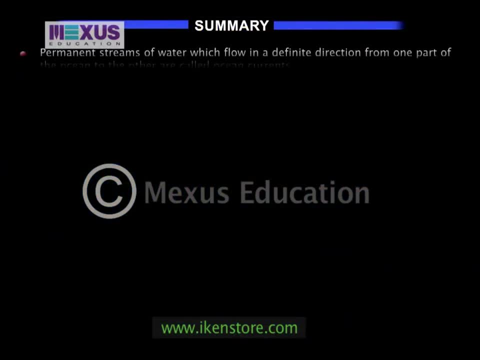 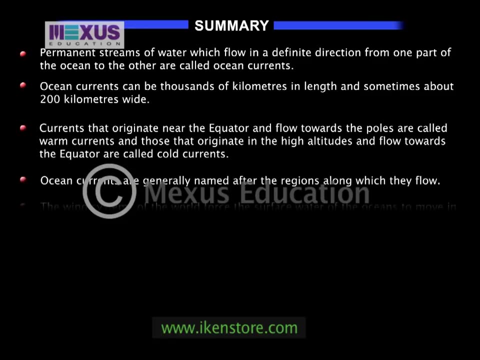 This always causestable change can result in thunderstorms. This is quite a think- perceber. The windузza asked is similar to the ocean waves, but those are not quite so strong winds. This is just the boat memorial to the San Juan, frankly.